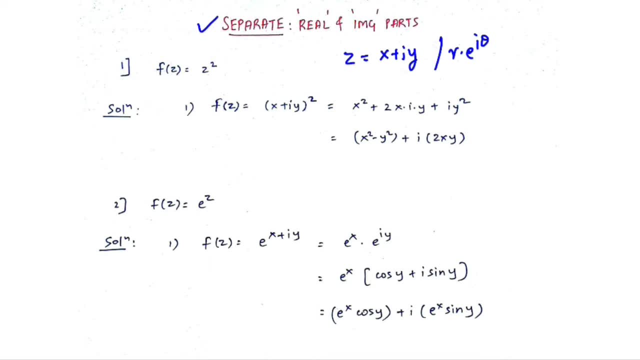 So here we are basically trying to separate the real and the imaginary part of a function. Now there can be various functions, so we will deal with varieties of quotient. Let us start with this first quotient f of z is given as z square. So if you replace this z by x plus iy, that is the rectangular form, you will get a plus b, the whole square format. Now you can open it as a square plus 2ab plus b square and after opening you have to know that you are collecting the real part here, like 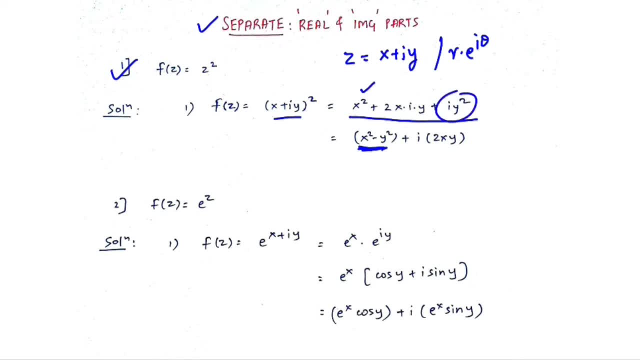 we have x square plus this. this. this part is iy, the whole square, which means it is minus y square, correct? So x square and minus y square are only the real part, whereas the imaginary part are plus i times 2xy. So here the real part is x square minus y square and the imaginary part is 2xy. So if you have understood about the separation of real and imaginary parts, tell me the answer for question number 2.. Now the question number 2 is f of z is given as e. 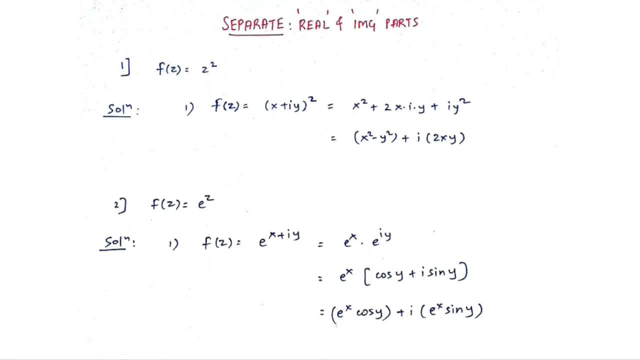 raised to z. So I hope you have tried once about solving this question, because again we are separating the real and imaginary part. what we have to do: replace this z by x plus iy. this means we are going for the rectangular form and now you can use your indices. if you have e raised to a plus b, according to the indices it is e raised to a into e raised to b. So now you can separate the terms and what you have to do. use the Euler formula. that is, e raised to i. theta is equal to cos theta plus i sine theta. 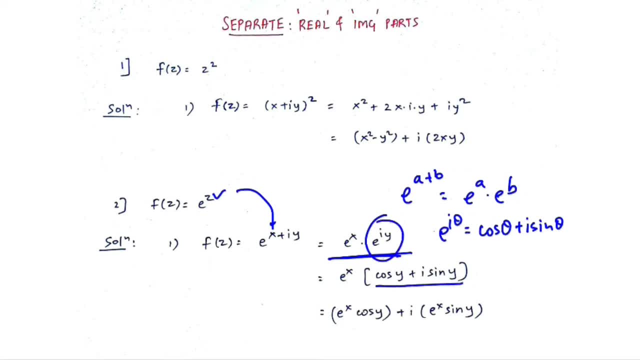 So, after doing the separation, this part would be changed to e, raised to iy would be changed to cos y plus i sine y. Now do the separation. this is the real part, this is the imaginary part, and you are done. This is all about the strategy. If, if, if you are reaching here but you don't know the Euler formula, you are gone. And if you know about this but you don't know about the indices, you are gone. So it's all about strategy. If you know the correct concepts, correct strategy, you can solve any question and that's it. 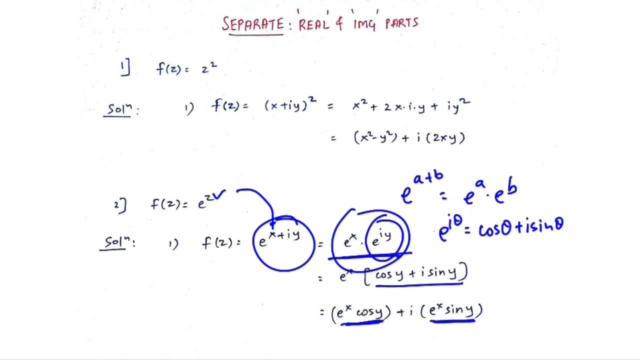 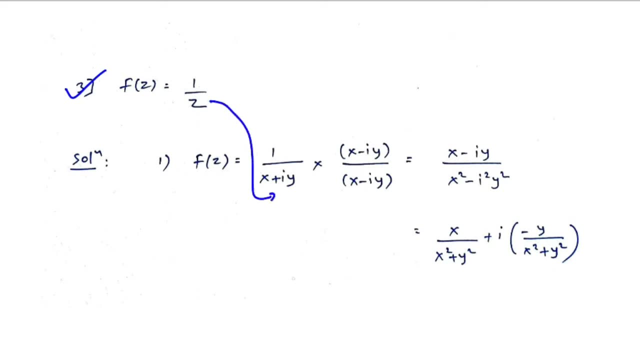 That's my guarantee. Now we will go for some tough questions. So the question number three is: f of z is given as one by z. Again, you can replace this z by x plus iy, no problem. but you cannot comment on the real and imaginary part. So what you have to do is we have to multiply, divide with the conjugate. So denominator has x plus iy. you are multiplying with x minus iy and dividing by x minus iy. Why you are doing this? What is the reason Why you are multiplying and dividing by the conjugate? 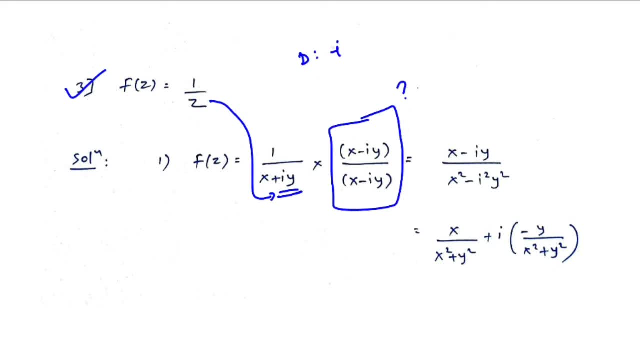 The answer is simple: In the denominator I have the complex part that is I. In the denominator I have I. I have to get rid of this. I So how I can get rid of Now. you can see that after doing the multiplication and division by the conjugate, Now the denominator is a plus b into a minus b format, which is a square minus b square. So do the math: It's x square minus iy, the whole square. You can say it is equal to x square plus y square. So now I am getting rid of the imaginary part that is the iy. 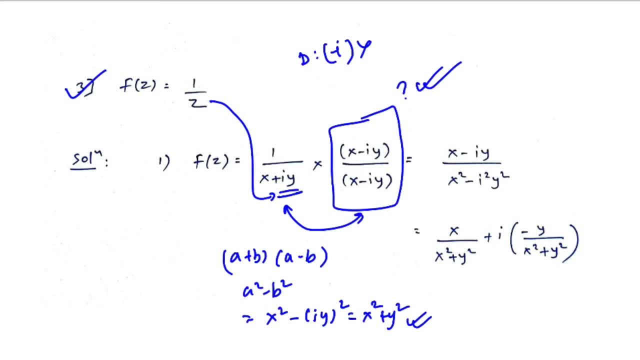 And that is the reason we are doing this technique, this operation. So, after doing the simplification, you can say x minus iy upon x square plus y square, which can be splitted as x by x square plus y square, and plus- i times this term- that is, minus y by x square plus y square. So this is the real part and this is the imaginary part. So I hope you got the good idea about how we can separate what techniques we have to use and let's go for some interesting questions as well. So this is example number one. 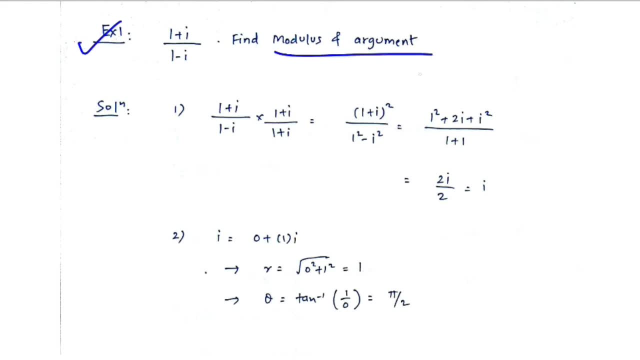 One plus i upon one minus, i Find the modulus and the argument. Modulus basically means they are going in the polar form, where r is the modulus and theta is the argument. Now you have to find these two terms. How you can find? First, you should separate. You should separate the real and imaginary part, because once you get the real part, that is x, and once you get the imaginary part, that is y, What you can say? your r is equal to root of x square plus y square and your theta is equal to tan inverse of y by x. 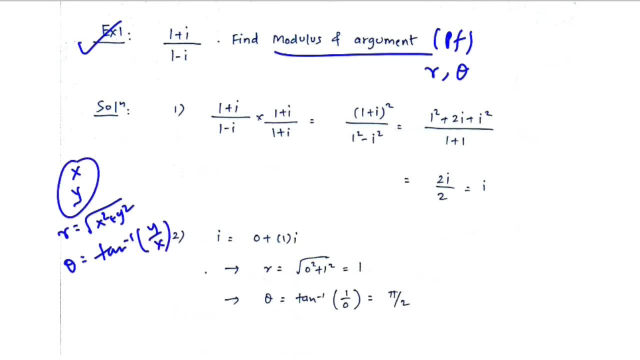 So I hope you are getting the idea why you need the real and imaginary part to get the answer. So first, what you can do is I want to get rid of this term. What I can do, I can multiply and divide by the conjugate. So now I am multiplying with one plus i, dividing by one plus i. Now this is a plus b, a minus b format which can be written as a square minus b square. Okay, After simplification I will get this term. Do the further simplification, you will get the value. as i Remember the iota is not. 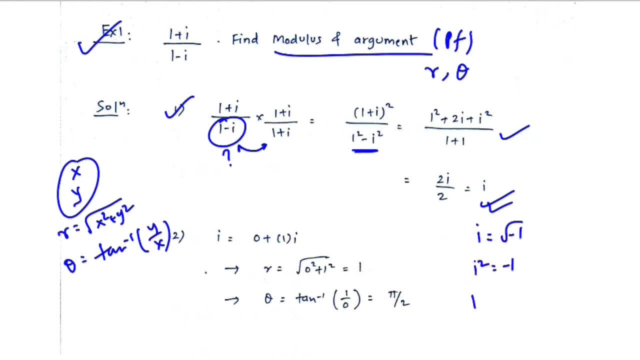 known as my root of minus one. So i square is minus one and i cube is minus i and i to the power four is one. So this much basics, this much idea you should have if you are doing the real and imaginary part, separation topic. So I hope you got the first step, that is, the value is i. Now the second step is i can be written as zero plus one times i. Why I am writing this? so that now I can say my x is zero and my y is equal to one. Now, once you get this, what's next? r? 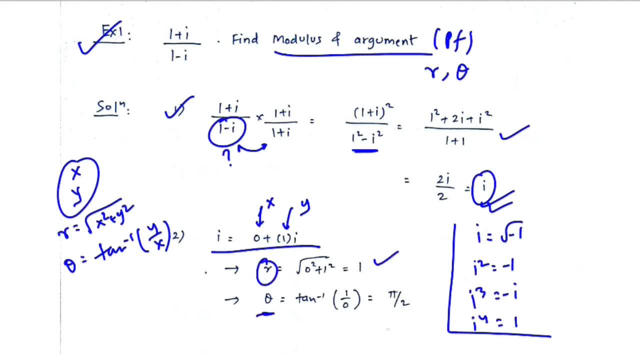 is equal to root of x square plus y square. So the answer is one: theta is tan inverse of y by x. The answer is pi by two. Now, this is pi by two, correct, because what is the reason? the x and the y terms are positive. You are in the first quadrant. That is the reason you are getting the answer is pi by two. But there is a homework for you. What if this x was negative? or what if this y was negative? Let us take this example: If x was positive and y was negative, Tell me what would be the value of theta. 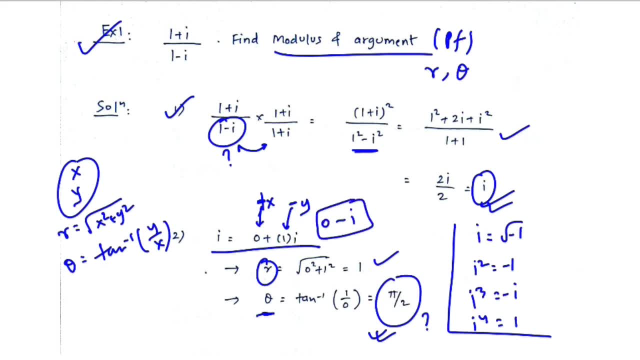 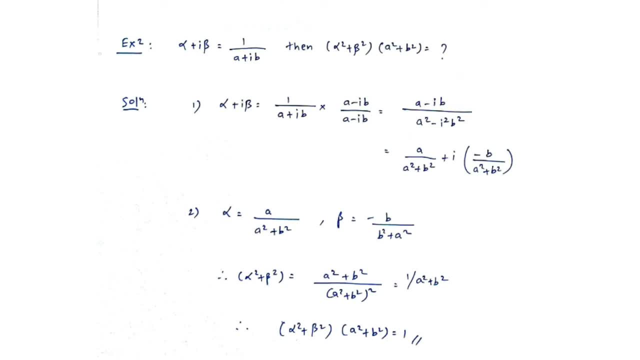 Okay, so the expression is zero minus i. If this was the expression, tell me what is the value of argument? Comment the answer. I will tell you whether it's right or wrong. So now we will see example number two. alpha plus i, beta is given as one by a plus ib. Then find the value of alpha square plus beta square into a square plus b square. Now it's simple, because up till now we have studied a good strategy on the separation of real and imaginary part. So what you can do is, first point, you have to get rid of this denominator which has 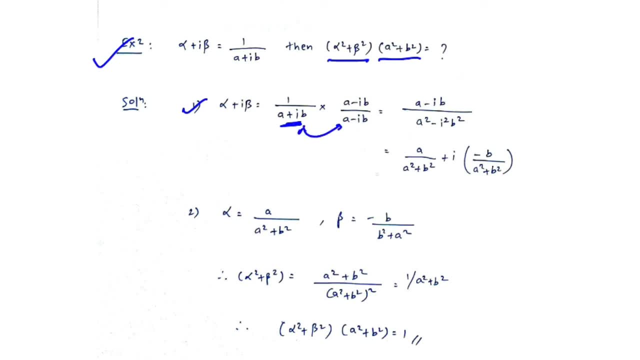 the iota term. So I'm multiplying, dividing by the conjugate, as you can see. So I'm getting rid of the denominator from the iota term. Okay, I'm not getting rid of the denominator, but the term that was present: iota, the term that was present, I'm getting rid of the iota. So that's it and you will get the answer. The real part is a by a square plus b square, and the imaginary part is minus b by a square plus b square. So now what you can say, your alpha- because now we have to equate this alpha- is this value and this: 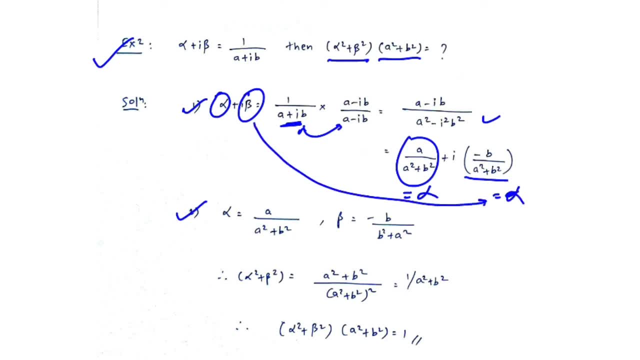 beta. this beta is this value, So this is beta. sorry, it's not alpha, it's beta. So alpha is a by a square plus b square. beta is equal to minus b by b square plus a square. Now, if you look carefully, what you need see, the question suggests you need alpha square plus beta square. So what you can do, 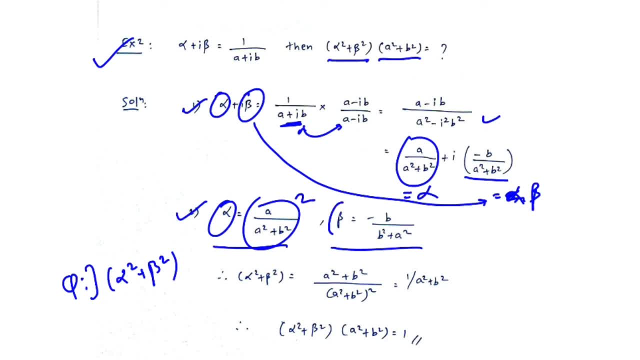 is you can square this term alpha square, So this would be squared, and you can square the beta part as well, So this would be square. Now you are doing alpha square plus beta square. you are getting the answer as a square plus b square upon a square plus b square, the whole square which can be written as 1 by a square plus b square. 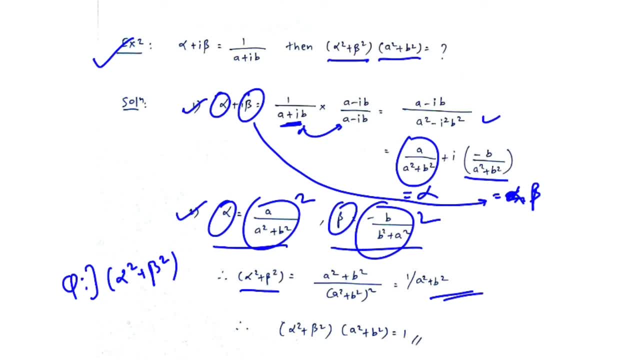 correct. Now, if you look carefully in the question, you need alpha square plus beta square into a square plus b square. Now do the rearrangement. you can bring this denominator in the left hand side, So alpha square plus beta square into a square plus b square. the answer is what? the answer. 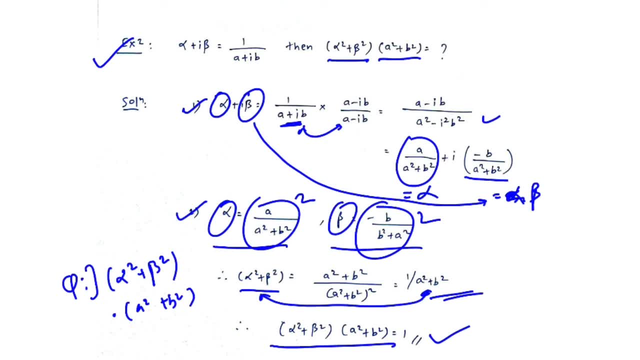 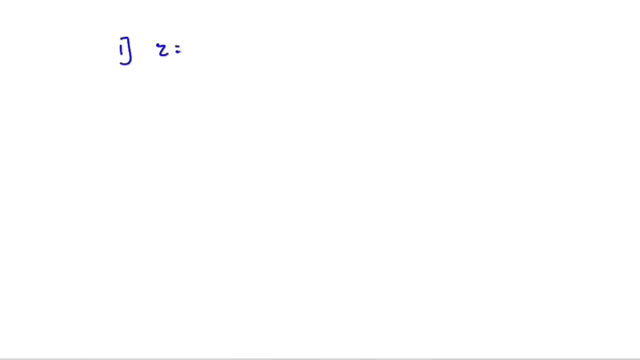 is 1.. So I hope you got the complete idea and I want to give some note so that you you are mastered in this topic now. So write some note. So the first point is z can be written as x plus iy in the rectangular form. So this is rectangular form. 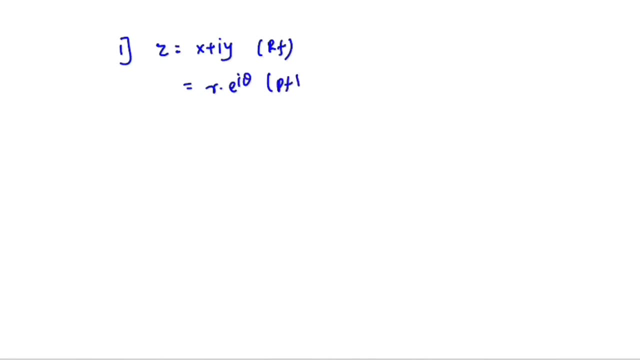 It can be written as r into e, raised to i, theta in the polar form. So r is equal to root of x square plus y square, the imaginary part square plus the real part square, correct, and the theta that is equal to tan inverse of y by x. So this was the basic everybody knew, because you have watched my. 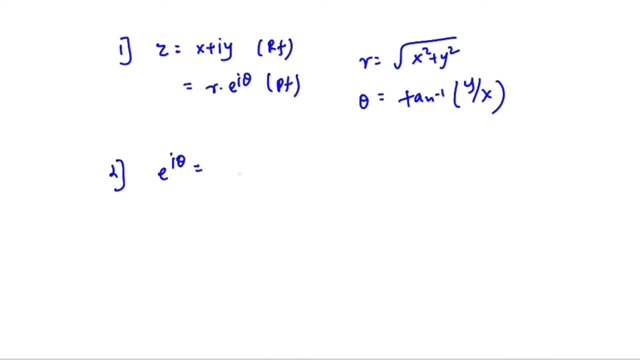 first video. Now the second point is your e raised to i theta. the euler form is cos theta plus i sin theta, And the second part, that is e raised to minus i theta is cos theta minus i sin theta. So you should have the knowledge of this as well. Also, you can write as if you have log of a, b, it is equal to: